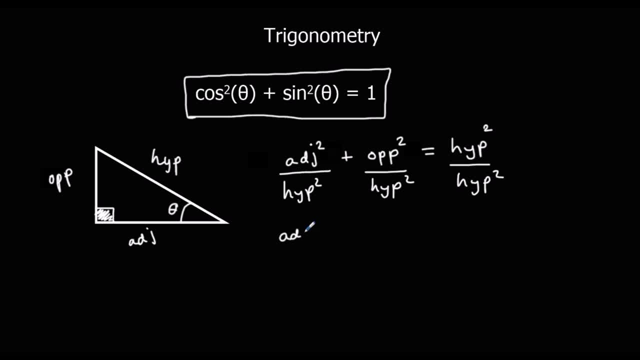 that give us. Here we've got adjacent over hypotenuse squared, Here we've got the opposite over the hypotenuse squared, And here we've got the hypotenuse over the hypotenuse squared, The adjacent over hypotenuse. 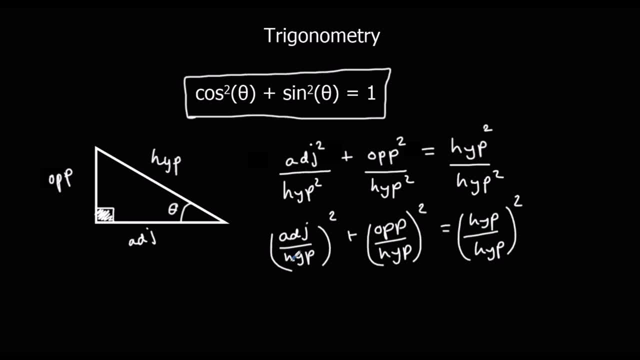 adjacent over hypotenuse is the same as cos theta, Because cos theta equals adjacent over hypotenuse. Sine theta is the opposite over hypotenuse. So we can change adjacent over hypotenuse to cos theta. I'll put cos? theta squared Opposite. 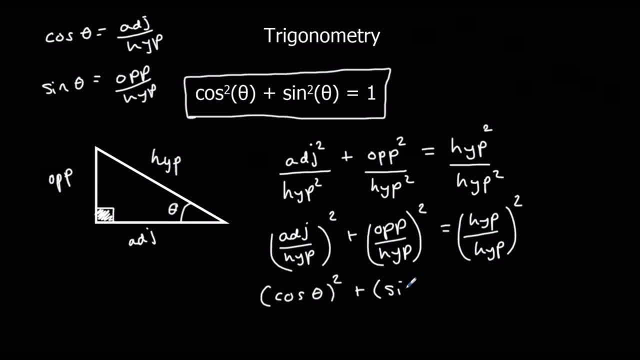 over hypotenuse. we're going to change to sine theta, So sine theta squared, And hypotenuse over hypotenuse. well, that's one, So I'll put one squared. Now we write: cos theta all squared as cos squared theta. 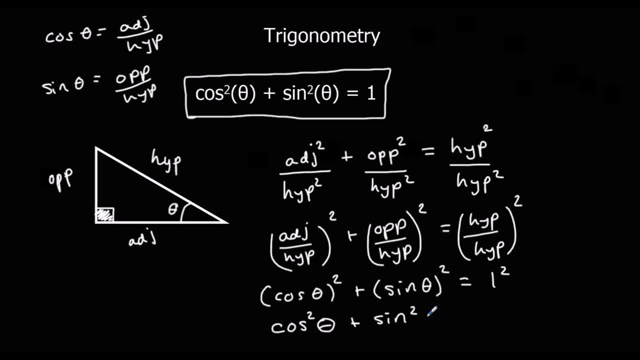 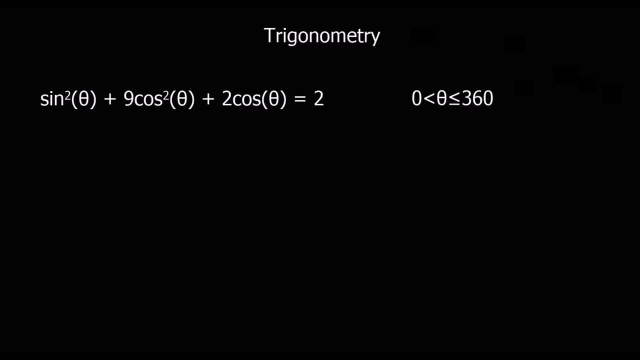 We write sine theta, all squared as sine squared theta, And one squared is one. So there we go. We've got our identity, cos squared theta plus sine squared theta equals one. So here we're going to look at a question that uses that identity. So we've got sine. 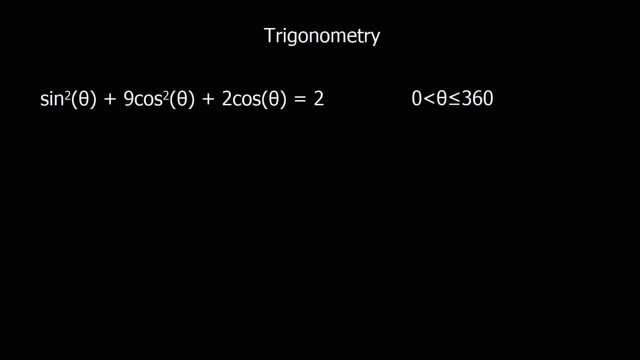 squared theta plus nine. cos squared theta plus two. cos theta is equal to two, And we're going to solve it for theta between zero and 360 degrees. so we're going to use this identity. so we're going to use cos squared theta plus sine squared theta equals one and we need to make it. 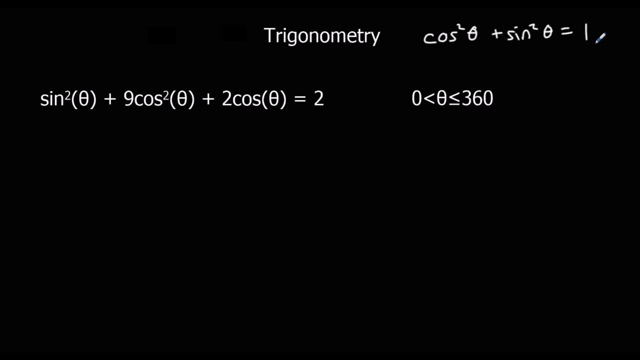 easier. so it's going to be a quadratic and to solve it we need it to all be in terms of cos or all be in terms of sine so we can solve it. so we need to either get rid of the causes or get rid of the signs. so the easiest thing to do, because i've got two cos terms here, only one sine term. 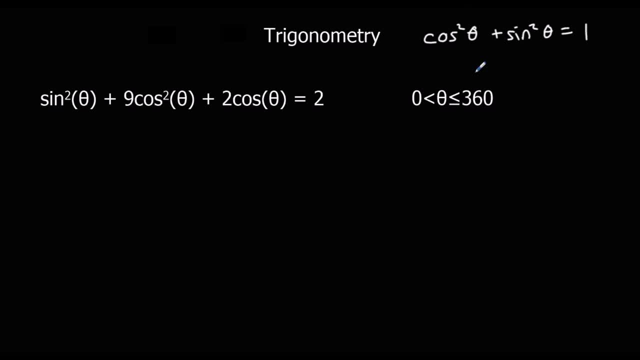 and the sine term is already squared, which makes it easy to use our identity. that's going to be the easiest thing to get rid of. so we're going to eliminate this term, the sine squared theta, And we're going to do that by substituting in what sine squared theta is equal to. 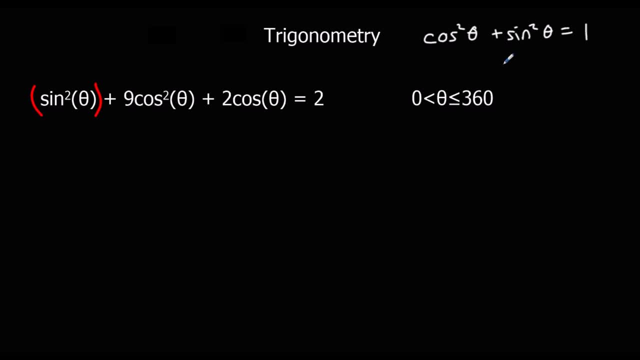 So if I subtract cos squared theta from both sides of the identity, So sine squared theta equals 1 minus cos squared theta. So I can substitute in for sine squared theta 1 minus cos squared theta. So I'm going to change sine squared theta to that. 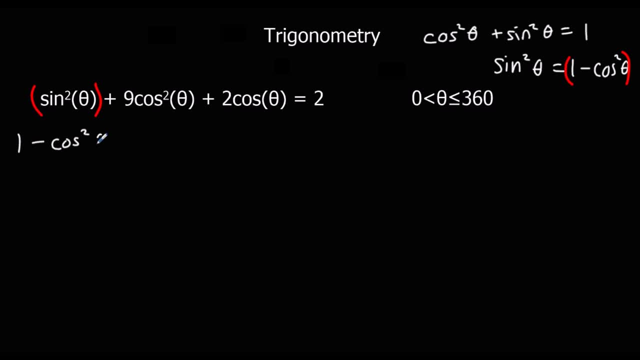 Which is going to give me 1 minus cos squared theta, plus 9 cos squared theta, plus 2 cos theta equals 2.. Now I'm going to collect the like terms. So I've got minus 1 cos squared theta, plus 9 cos squared theta. 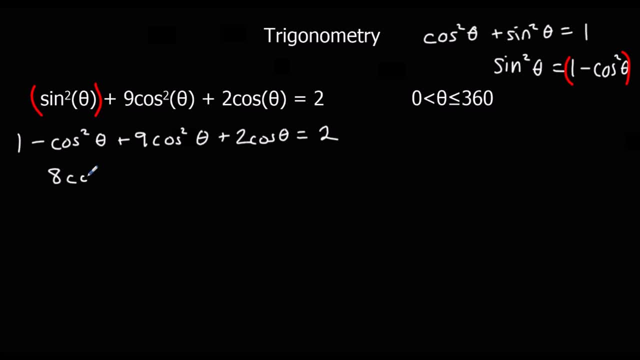 So that's going to be 8 cos squared theta Plus 2 cos theta, And I need to make it equal to 0 to solve it. So I'm going to subtract 2 from both sides. So 1 take away 2.. 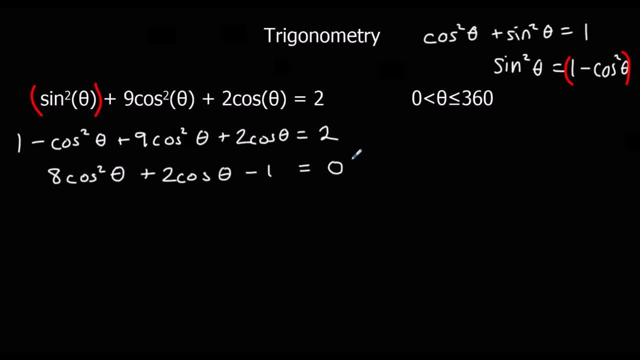 That's minus 1.. So now I've got the normal quadratic equation. So I could use the quadratic formula, Or I could factorise it, Or I could complete the square. Whichever method you want to use, I'm going to factorise this. 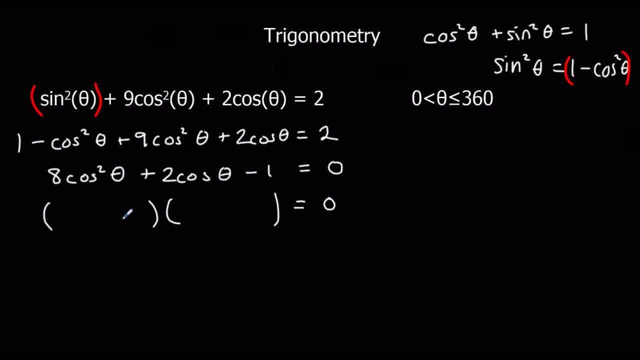 So I've got the only thing that multiplies to make 1 is going to be 1. And I'm going to have to make 2 cos theta. I'm going to have 4 cos theta and 2 cos theta, And I want the 4 to be positive and the 2 to be negative. 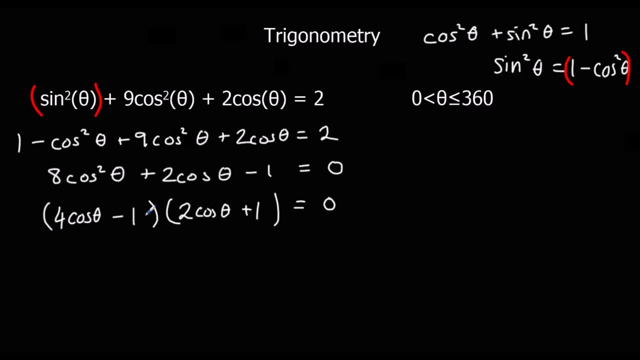 There's lots of ways of factorising. If you use a different method, that's okay, As long as you get the same answer. If you use the quadratic formula, that's okay, As long as you get the same answer. So the answer should be: cos theta equals a quarter. 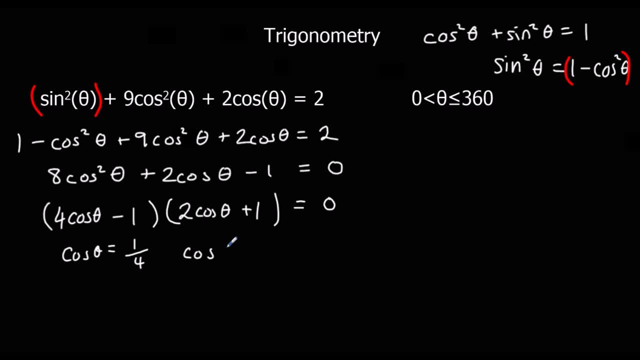 Because that's what makes this first bracket 0. And cos theta equals minus a half, Because that's what makes the second bracket 0. So we need to solve now. So we need to make sure the calculator is in degrees, Because we need the answers between 0 and 360 degrees. 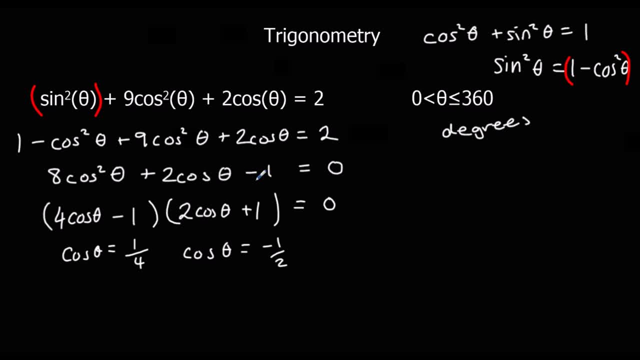 And to get theta by itself, we're going to shift cos. So shift cos 1 quarter first. So type that into the calculator: Shift cos 1 quarter And we should get 75.5 degrees to 1 decimal place. To get the next answer for cos we do 360 minus answer. 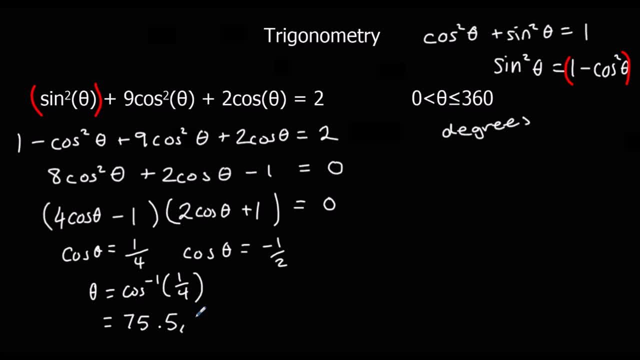 So 360 minus the answer, 284.5.. So there's two answers. Now we're going to work with this. Cos, theta equals minus a half. So to get theta by itself, shift cos minus a half this time And that should give you 120 degrees. 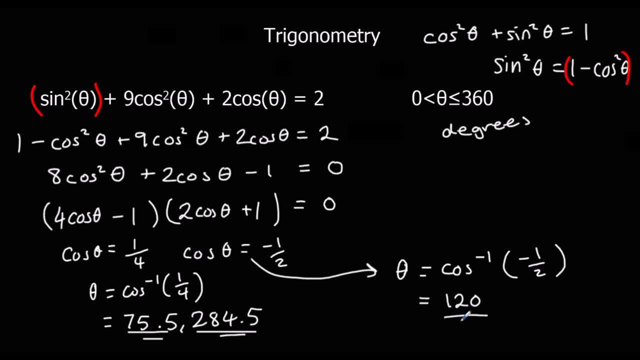 And 360 minus answer: Well, that's 240 degrees. So we've got four answers there. We can't get any more answers Because if we plus 360 or take 360 from any of these, it'll go out of the range we wanted. 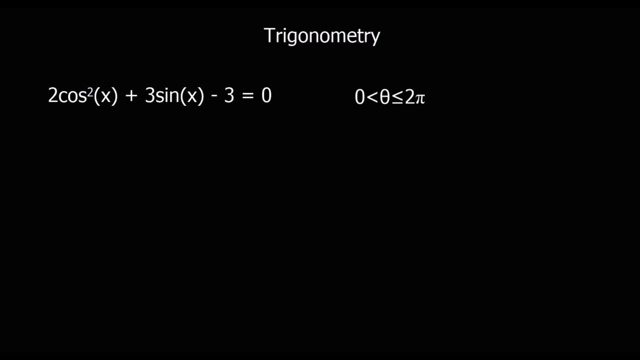 So there's our four answers. Okay, here's another question. You can pause the video and give it a go if you like, Or you can just carry on watching. So we've got 2 cos squared, x. So in x. this time this should say x. 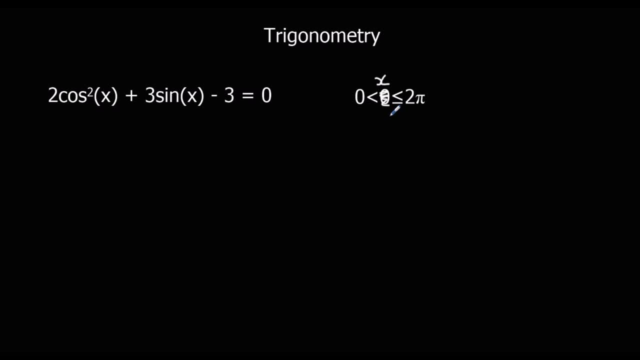 Doesn't make a difference to the question 2. cos squared x plus 3, sin x minus 3 equals 0. And we want the answers for x between 0 and 2 pi. So we're going to be in radians And we're going to use our identity. 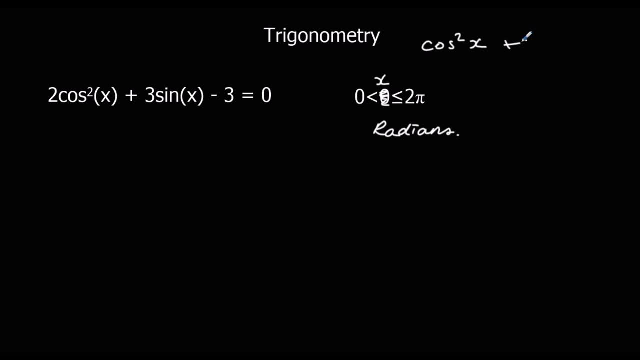 Again: cos squared x plus sin squared x. Cos squared x Equals 1. To solve this equation. So what's easier to get rid of? Is it going to be the cos or the sin? Well, the cos is squared, So that's going to be easier to get rid of. 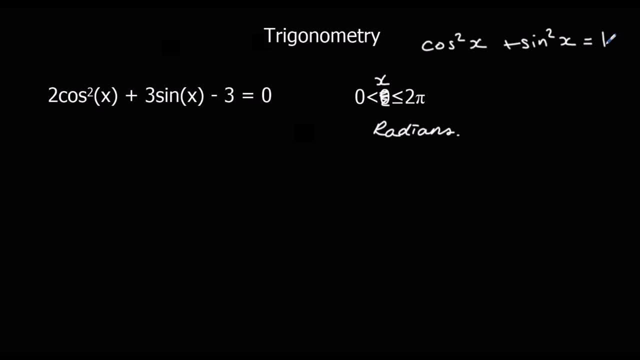 We could get rid of the sin, But it'll be a lot harder. So the easiest thing to do would be to substitute in for cos squared x. So cos squared x Is equal to 1 minus sin squared x. So we can just substitute it in. 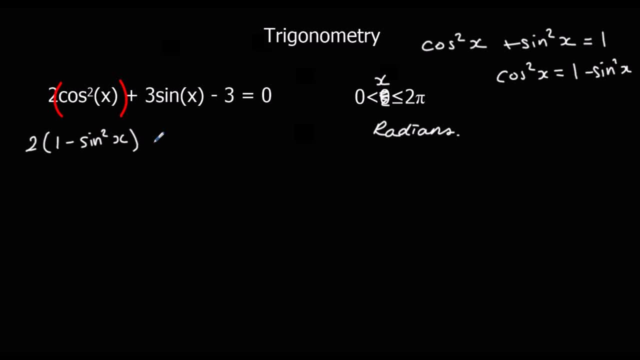 1 minus sin squared x, instead of cos squared x. And then we're just going to simplify, So we're going to expand the bracket, So multiply it by 2.. So that gives me 2 minus 2 sin squared x Plus 3 sin x. 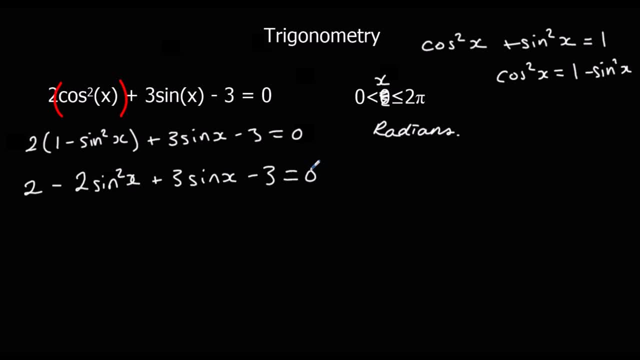 Minus 3 equals 0.. Collect like terms. So we're going to have minus 2 sin squared x Plus 3. sin x 2 minus 3 is minus 1. Equals 0. I don't like the first term being negative. 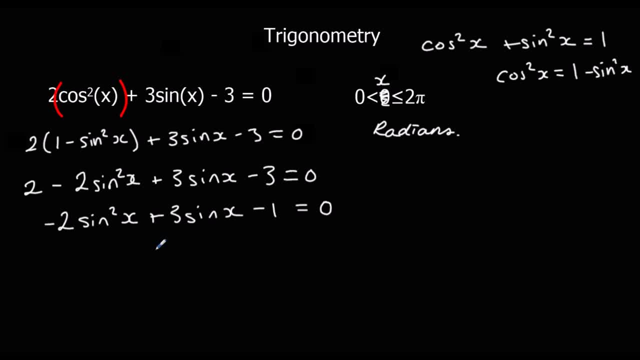 So I'm going to multiply everything through by minus 1.. So that will give me 2 sin squared x Minus 3. sin x Plus 1 equals 0.. And again we've got the familiar looking quadratic equation. So we could factorise or use the formula. 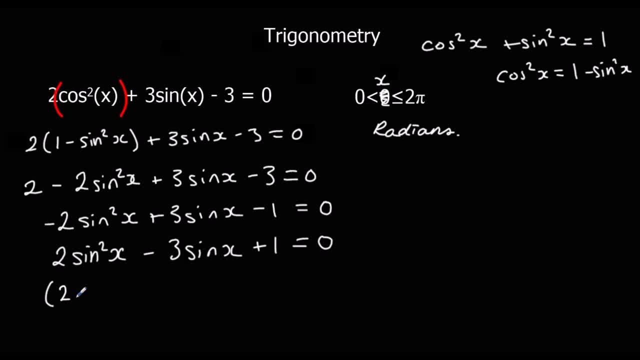 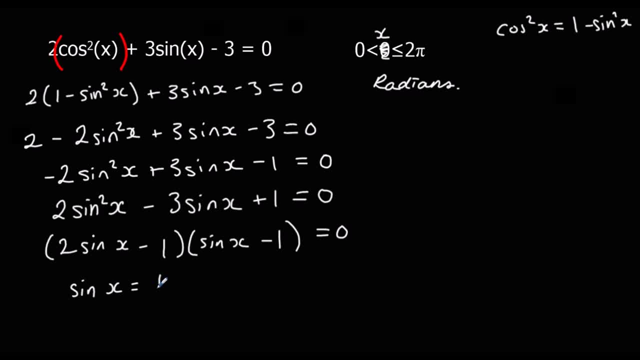 Minus, Minus, Minus, Minus, Minus, Minus, Minus. What makes the first bracket 0?? So sin x is a half. Or what makes the second bracket 0?? Sin x is 1.. 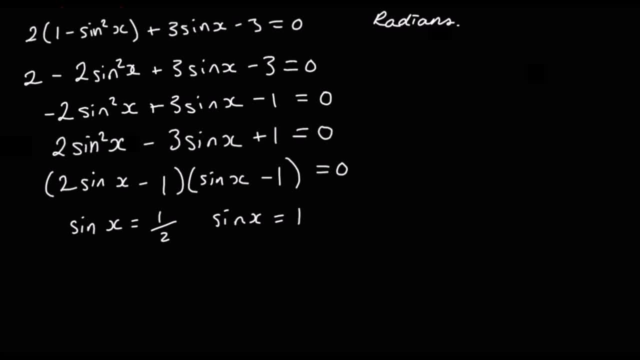 So to get x by itself, we're going to shift sign Making sure the calculator is in radians. So shift sign a half And that's going to be shift sign a half, Which is going to be 1, sixth pi. and to get the next answer in for sine, we do pi minus answer. so that's going to 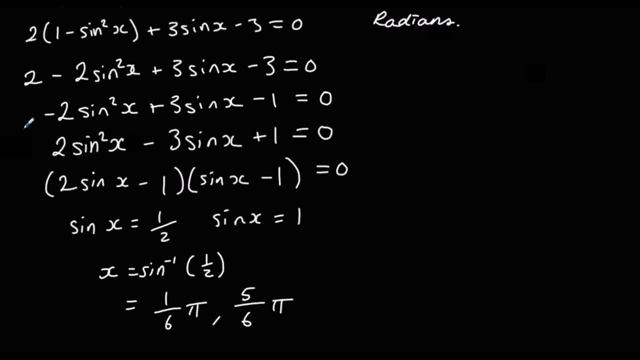 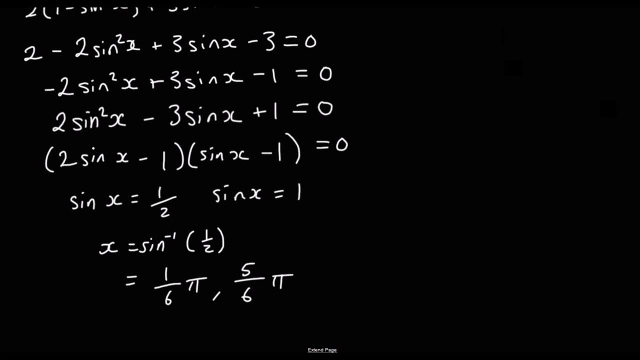 be 5, 6 pi. both those answers are within the range we wanted and I can't get any more, because if I add 2 pi to these they'll be over 2 pi. so there's two answers there and then we're going to shift sine 1. so shift sine 1, that should. 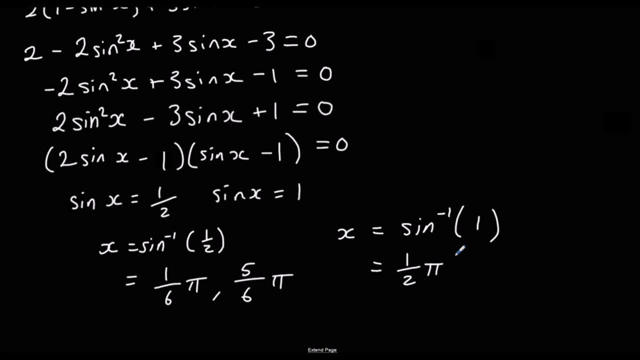 give us half pi and, interestingly, if we did pi and minus answer to try and generate another answer, we're going to get half pi again. the reason is: do a quick sketch. so here's the sine wave. sine is only one at one point. it's the maximum, it's the peak, so it's only one. 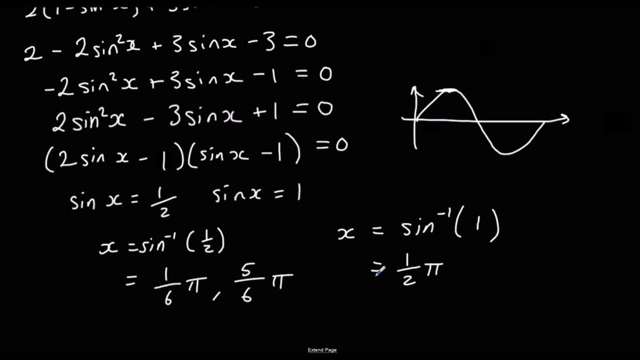 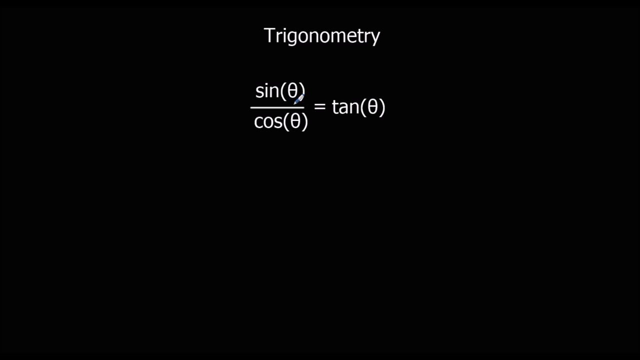 at one point in a 360 degree cycle. so we've only got one answer. so in total we've got three answers for this. we've got 1, 6 pi, half pi and 5, 6 pi. okay, here's another trigonometric equation: 2 times 4 pi raised to 16, sì, 2 pi over 2 esa output. 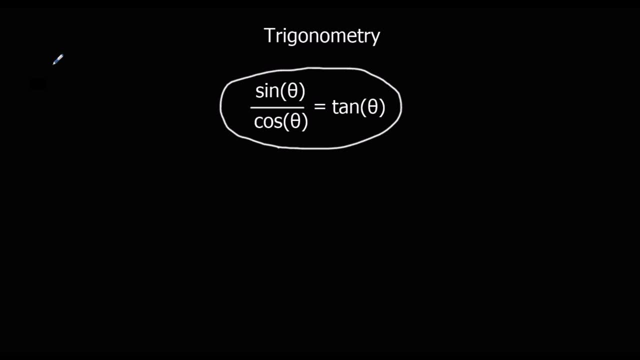 everything that we have or I put in here. it's only one answer, so we need to solve, and I have to solve. it's only one rule we need to solve. it's only one problem, so we make it one, because we need one instruction or we need another. 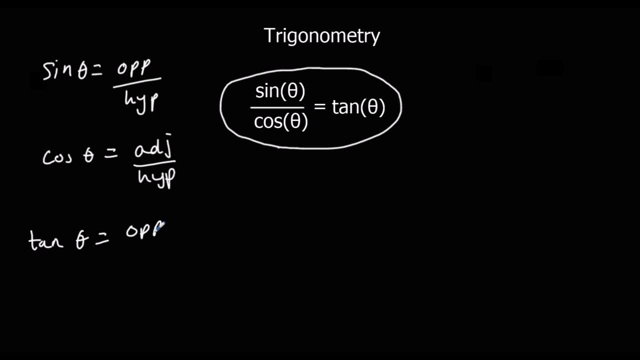 we need two. extracting these. here we have 4 pi and a sine sine theta. our formula be seen after the left over cosine theta. it increases trans婶 opposite over adjacent. So if we take sine theta and divide it by cos theta, that means 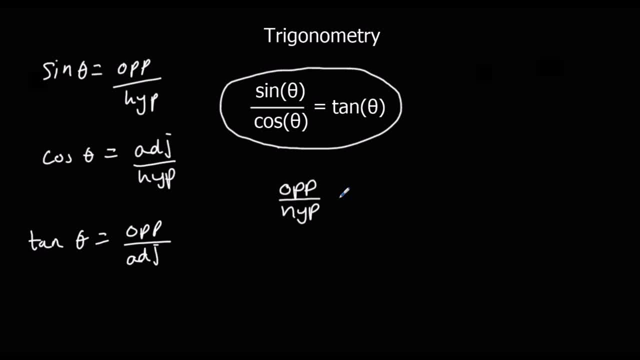 we've got opposite over hypotenuse. divide by adjacent over hypotenuse. If we're dividing a fraction, we can change it to a times and flip over the second fraction, And then we're going to cancel off the hypotenuse, which is just going to leave us with opposite over. 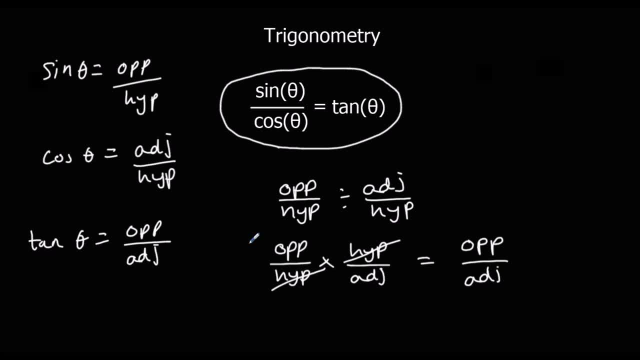 adjacent, which is tan, which is tan theta. So if we divide sine theta by cos theta, we get tan theta. So sine theta over cos theta is tan theta. Now we're going to look at an equation where we're going to use that identity. 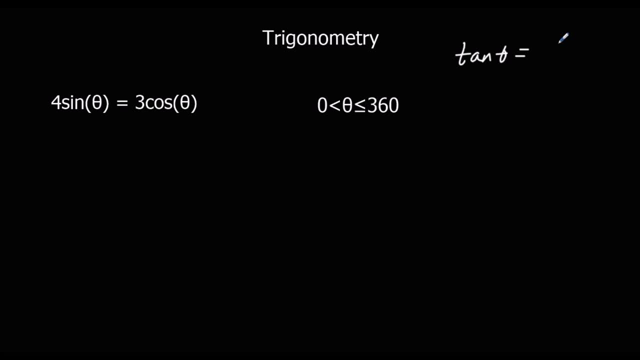 So we're going to use tan theta is sine theta over cos theta, So we're going to solve this, for sine theta equals 3 cos theta for theta between 0 and 360, so degrees. How can we use this identity? We just need to divide through by cos theta. So if you divide both, 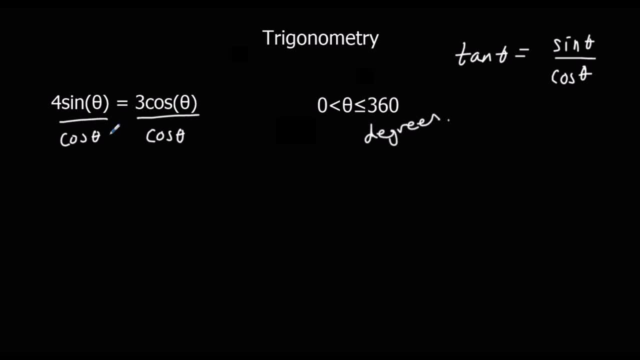 sides we've got a cosine theta over cos theta, So we're going to use tan theta. So that's 4 tan theta. And on the right side you've got 3 cos theta over cos theta, And cos theta over cos theta is 1.. Anything divided by itself is going to give us 1.. So we've just got 3. 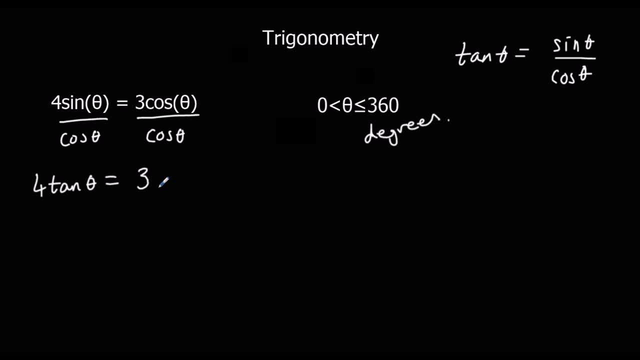 left, on the left side. So we've got 3 cos theta over cos theta, which means we've got two cos theta And we're going to put those two cos theta. So we'll just divide by 1 over right side. now you want to get 10 feet by itself, so we're going to divide both. 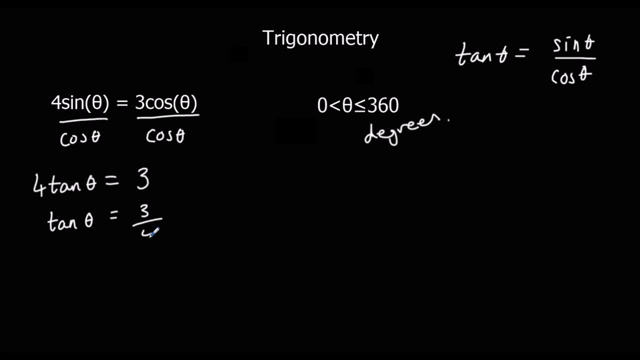 sides by the 4, so 10 feet are equals 3 quarters. and to get feet by itself will you arc tan. so shift tan 3 quarters. so in the calculator shift tan 3 quarters and that should give us thirty six point nine to one decimal place. and to get the 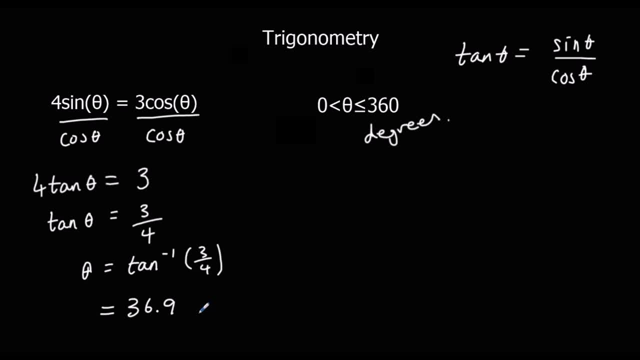 next answer for tan. we just add on 180 and that's two hundred and sixteen point nine degrees. so we've got two answers between zero and 360, and there are answers okay. so here we've got another question using the same identity. so we're going to use the identity that. 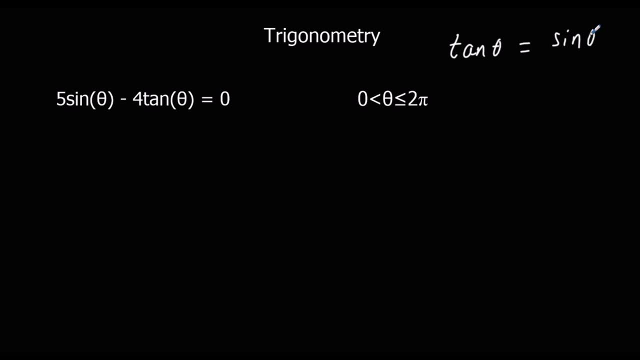 tan theta equals sine theta over cos theta. so we've got a question. it says 5 sine theta minus 4 tan theta equals 0 and we need the answer between 0 and 2 pi so you can make sure I calculate some radians. so in this instance we're going. 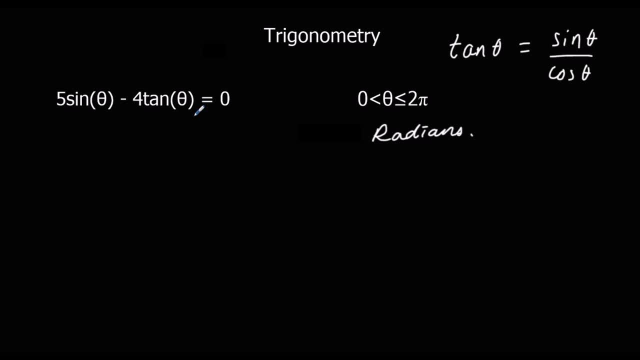 to substitute in for tan theta. so we're going to change tan theta to sine theta over cos theta. there's nothing else we can do, so that's going to be where we start. so we've got 5 sine theta minus four sine theta over cos theta equals zero. now we're going to multiply through by cos theta. I'm going 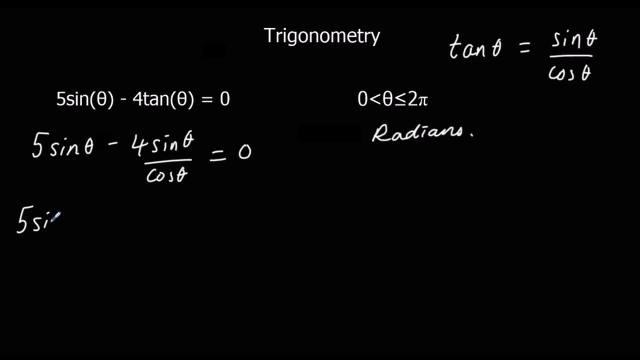 to get everything on the top. so that's going to give us five sine theta cos theta. if I multiply by cos theta I cancel out the fraction. so that's just 4 sine theta and 0 times cos theta is still 0. now it would be tempting here to divide through by sine theta. 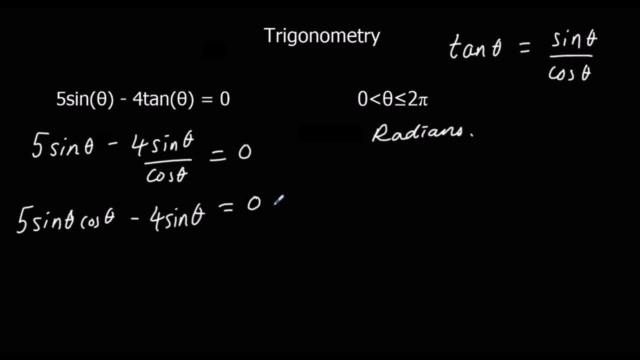 and eliminate it, get rid of it. that isn't what we want to do. that would lose us some answers. so instead of dividing through by it, we're going to factorize it. so we're going to take sine theta outside the bracket, which is going to leave us with 5 cos theta minus 4 inside the bracket. 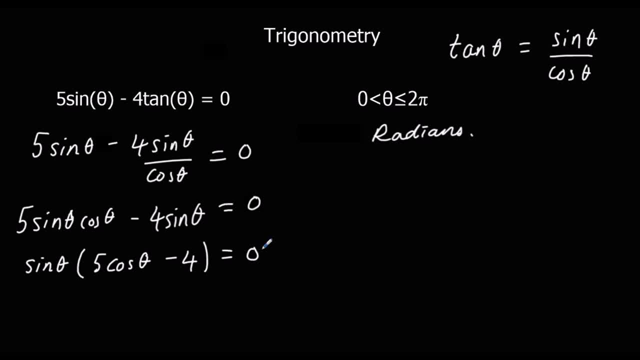 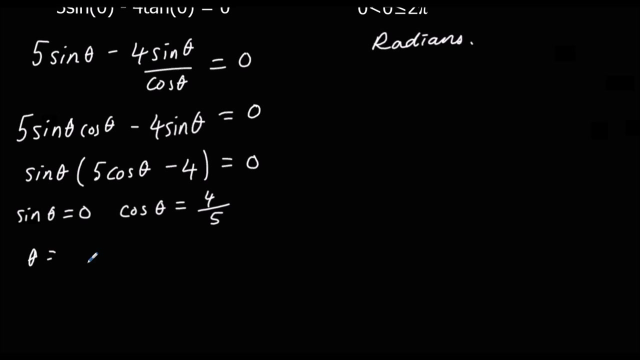 so what are the answers we can have? either sine theta equals 0 or cos theta equals 4 fifths. so now we're going to to solve, we're going to shift sine and shift cos. so theta equals shift sine of 0. so shift sine 0 gives us an answer of 0.